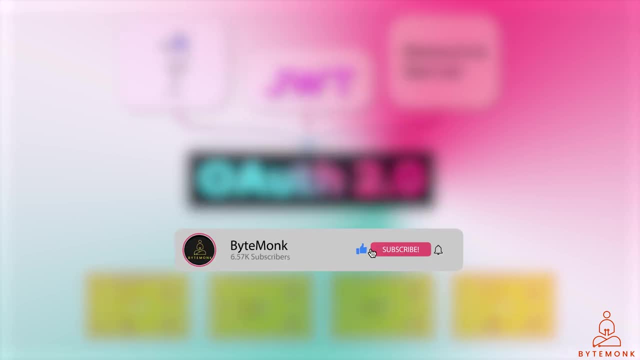 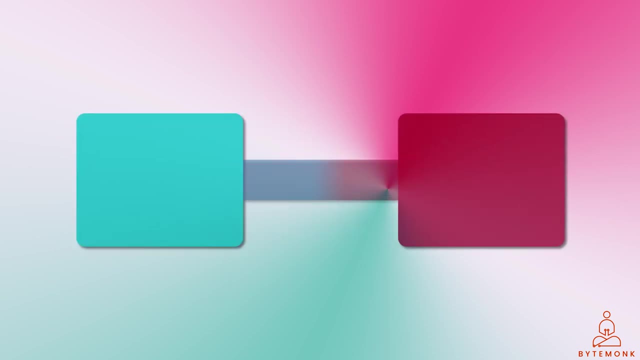 a cornerstone for modern digital security. So let's dive in. Simply speaking, OAuth 2.0 is a way for two websites to talk to each other without sharing your password. It works like this: Let's say you want to play a game on your computer. 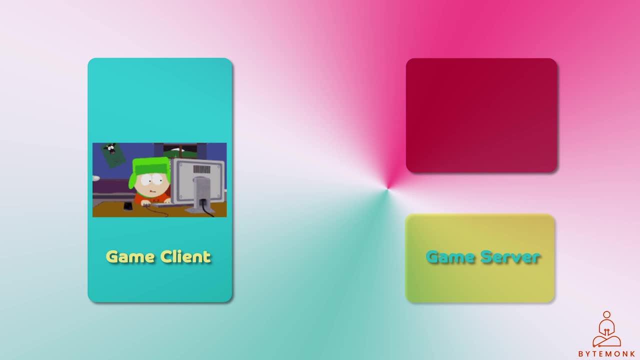 but you need to log in to your Google account to play it. You don't want to give the game your password, So you use OAuth 2.0 instead. The game websites ask you to log in to your Google account. You go to Google and log in. Google gives the game's website a special code. 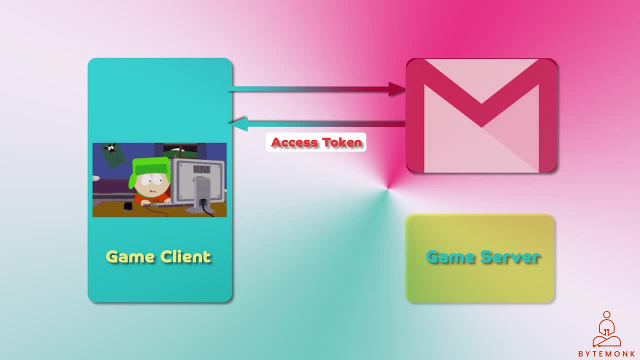 called access token. The game website uses the access token to talk to Google and get your data, And then you can play the game. The access token is like the key that lets the game website talk to Google on your behalf. It is a short-lived credential that allows an application to access a user's 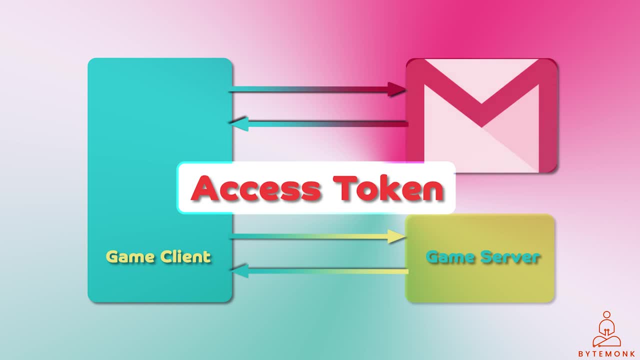 account by sharing an account with the user. It is not the user's password and it does not grant the application full access to the user's account. The access token is typically generated by an authorization server after the user has granted the application permission to access their resources. The authorization server. 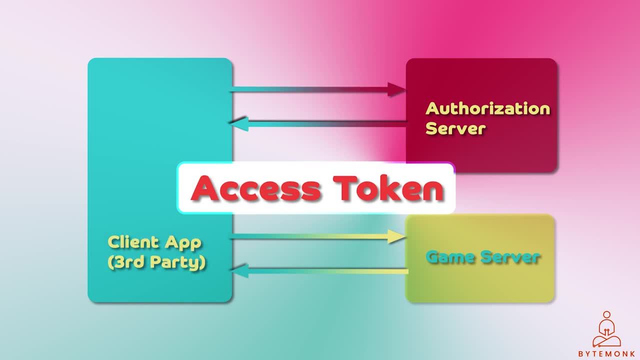 then returns the access token to the application, which can then use it to make requests to the resource server. The access token is typically used in conjunction with the authorization header which is added to each application. For example, for the authorization header, it is added to the. 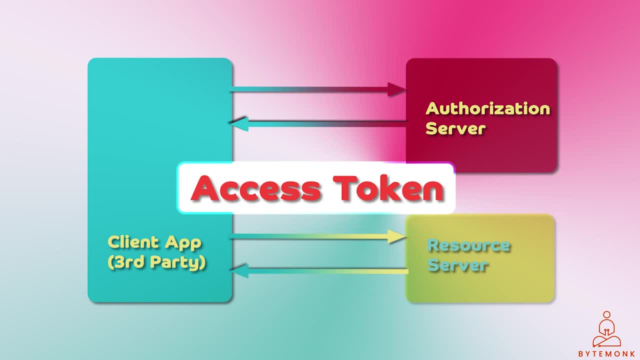 request made to the resource server. The authorization header includes the access token as well as the type of the token, for example bearer token, and the token's expiration time. The resource server then validates the access token and, if it is valid, grants the application access to the requested resources. 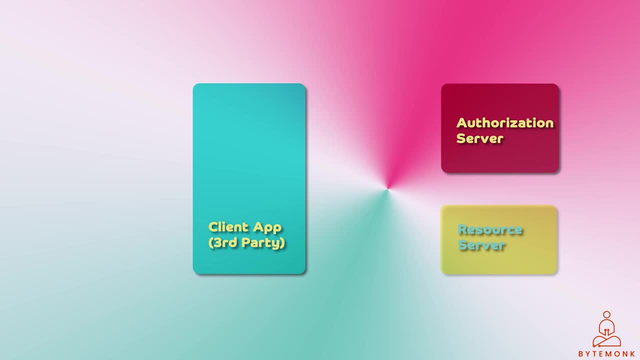 Here is an example of how an access token is used in the OAuth 2.0 authorization code flow. The user visits the application website and clicks on a button to log in with Google. The application redirects the user to the Google authorization server. The Google authorization server asks the user to log into their Google account. 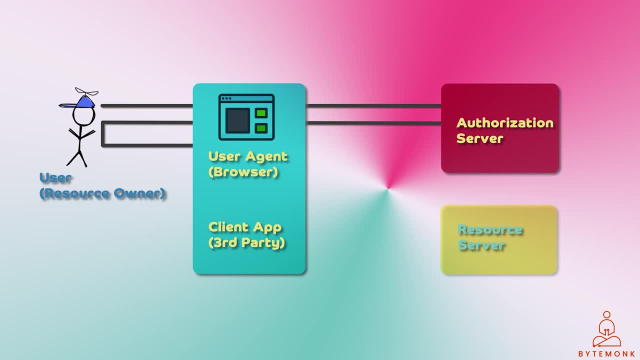 The user enters the username and password and clicks the allow button, The Google authorization server generates an access token and redirects the user back to the application's website. The application receives the access token and stores it in its database. The application uses the access token to request to Google's API. 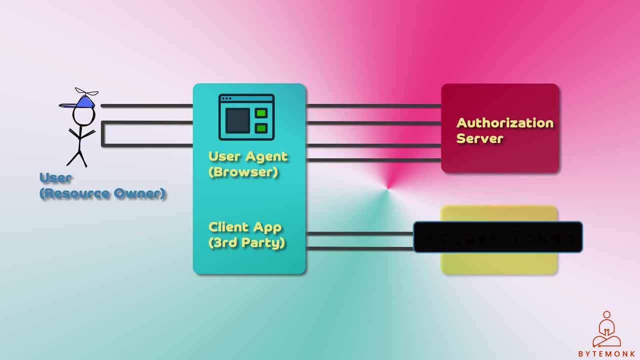 The access token is then suf yêu𝒚. JP web token is only valid for a certain amount of time, after which it expires. When the access token expires, the application will need to obtain a new one from the authorization server. Access tokens are an important part of the OAuth authorization framework. They allow applications. 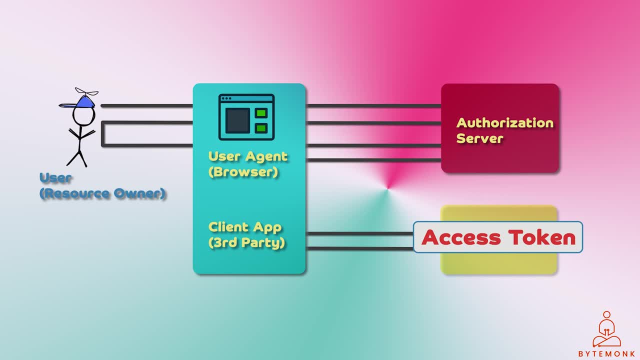 to access protected resources on behalf of users without having to share the user's password, and this helps to protect the user's privacy and security. The resource server is not explicitly mentioned in the flow, but it is the entity that hosts the protected resources that the application wants to access. In the example above. 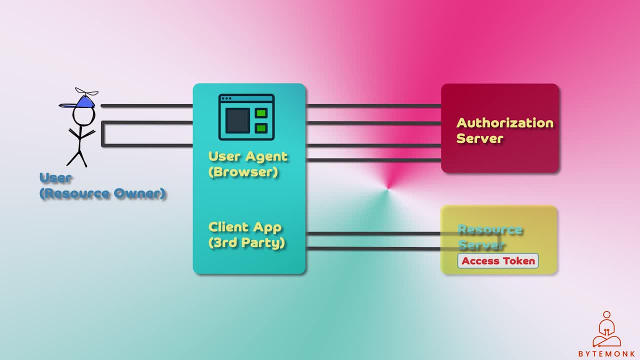 the Google APIs are the resource servers. The resource server is not involved in the authentication or authorization process. It simply validates the access token and, if it is valid, grants the application access to the requested resources. The resource server can be implemented in different ways depending upon the specific use. 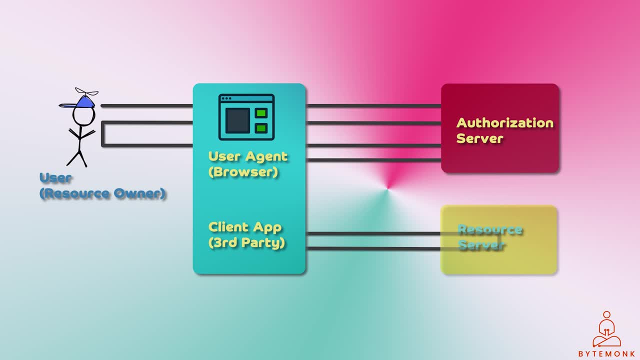 case. For example, the resource server can be a web application, a mobile application or a cloud service. Now I have covered JWT in detail in my previous video. If you are interested in learning more about JWT, please subscribe to my channel. 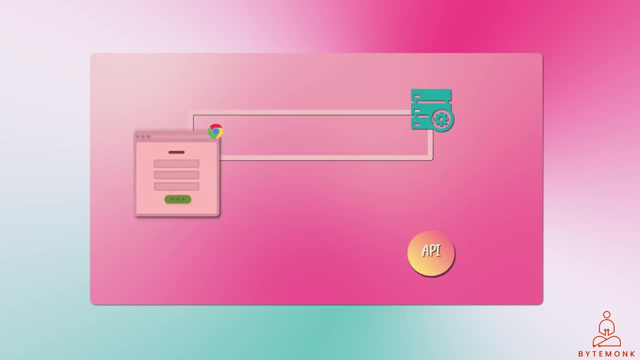 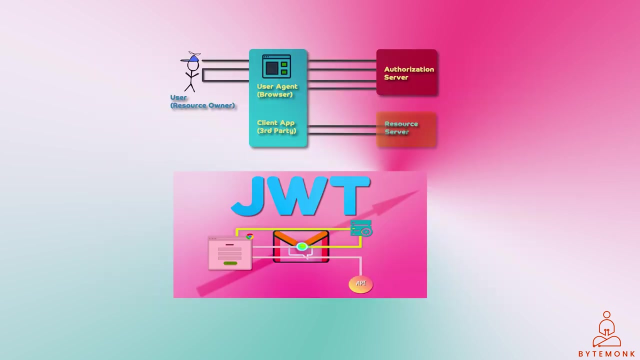 In this video I explained how they are a great way to authorize users and perform role checks in front-end to back-end communication and in distributed microservices architecture. OAuth 2.0 and JWT are two different protocols, but they can work together to provide a secure 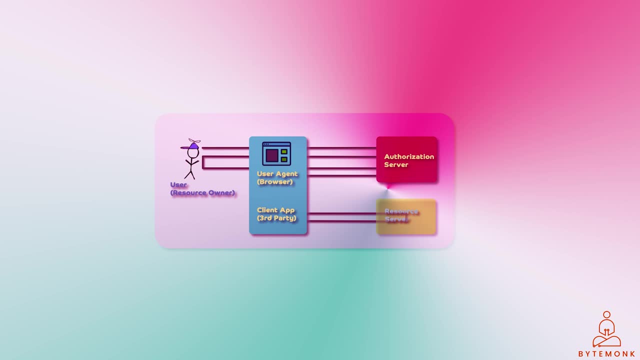 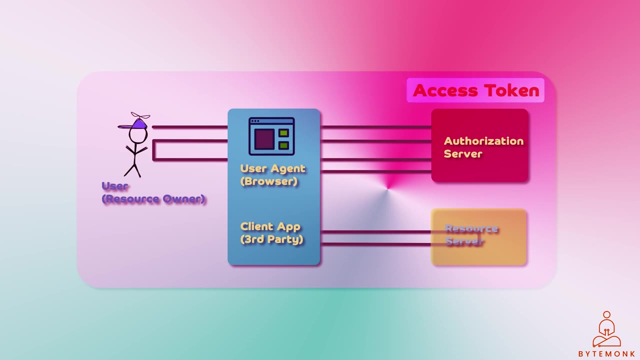 and efficient way for third-party applications to access protected resources. In the context of OAuth 2.0, JWTs can be used to represent access tokens. This is because JWTs are self-contained and can be easily verified by the resource server. Let's say you want to use a third-party application to access your Google Calendar. 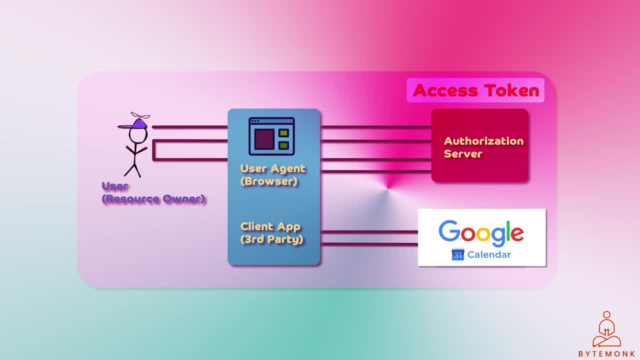 The third-party application first needs to obtain an access token from Google. It does this by using OAuth 2.0 to authenticate you with Google. Once you have authenticated, Google will issue an access token to the third-party application. The third-party application then takes the access token and encodes it as JWT. 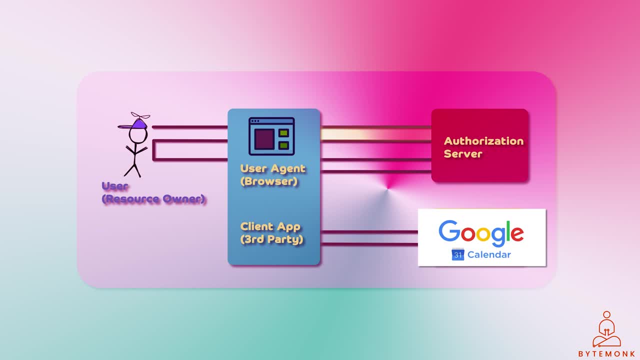 The JWT is then sent to the resource server, which is Google Calendar in this case. The resource server can then verify the JWT and grant the third-party application access to your calendar. The use of JWTs with OAuth 2.0 provides a number of benefits. 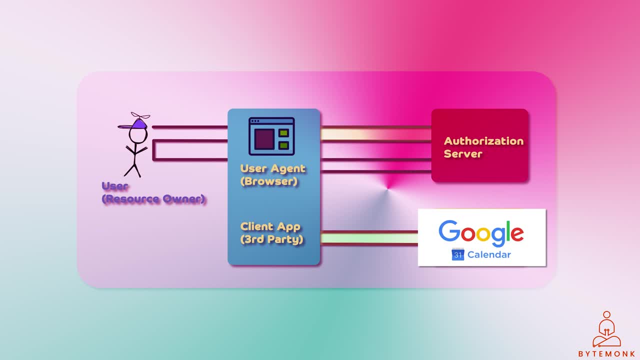 JWTs are self-contained and can be easily verified by the resource servers, and this makes them more secure than other types of access tokens, such as opaque tokens. JWTs are also compact and URL-safe, making them easy to transmit over the network. 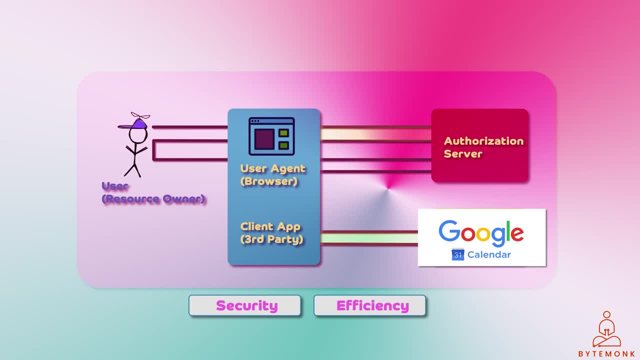 and this can improve the performance of OAuth 2.0 applications. The third-party application can then verify the JWT and grant the third-party application access to your calendar. The use of JWTs with OAuth 2.0 can then verify the JWT and grant the third-party application access to your calendar. 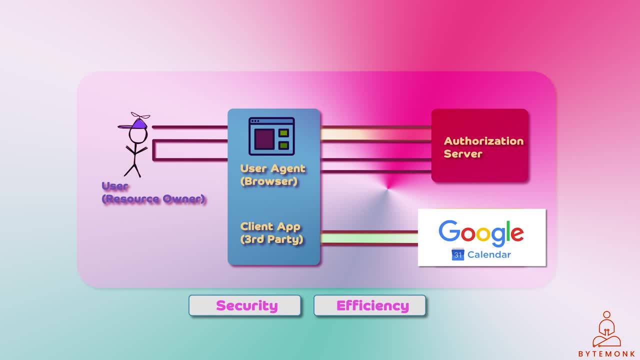 JWTs can be used to represent a variety of claims, such as identity, authorization or other data, and this makes them versatile and adaptable to different use cases. Overall, JWTs are a lightweight token format that can be used to transmit authorization information. 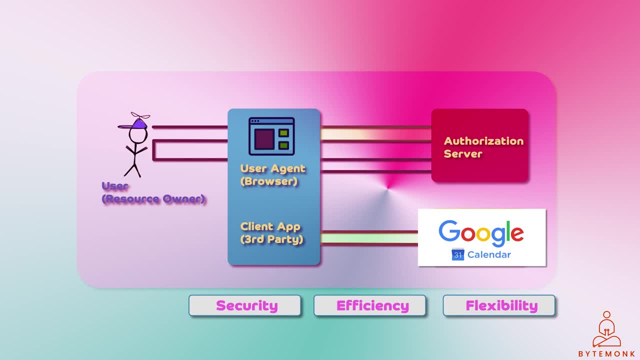 but they do not provide any authentication or authorization services themselves, Whereas OAuth 2.0 is an authorization framework that can be used to authenticate users and grant them access to protected resources. Overall, OAuth 2.0 and JWT are two powerful protocols that can be used together to provide a secure 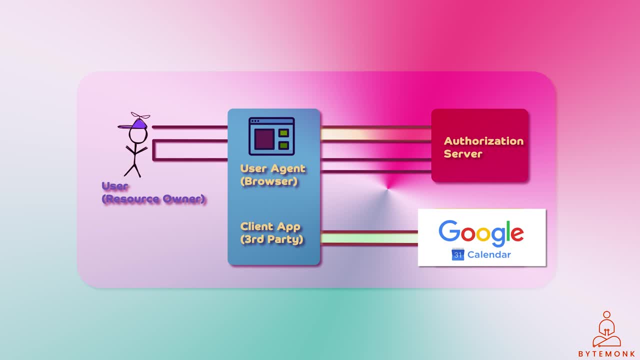 and efficient way for third-party applications to access protected resources, also known as SSO or Single Sign-On. In the example above I gave, the Google Authorization Server is also a Google Identity Provider. It is the entity that authenticates the user and issues the access. 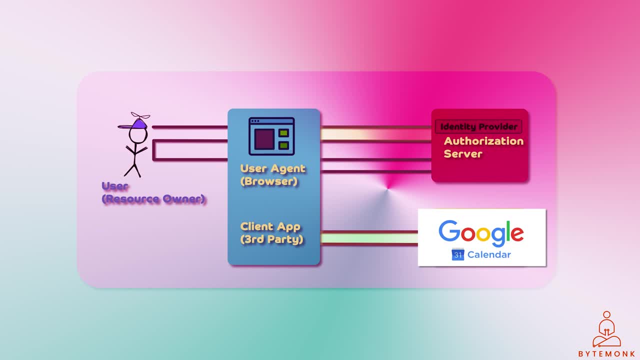 token, This is because Google is large, a trusted organization that can provide both authentication and authorization services. However, in other cases, authorization server and identity provider may be separate entities. For example, a company might use a third-party identity provider to authenticate it users and then use engines. Given that third-party authentication company might use an authorised server and identity provider to authenticate users. Also, the use of 3rd-party authentication and identity providers is, at the same time, most likely to receive additional afforded users, for example, to authenticate a Server or identity provider, such as a authentication server or authorization contact. The492. Number 5 is Authorization Server and Identity Provider- The492. This citrus topic includes opportunities forневutet 오늘 that there are several differences In it. we believe thatround Parallel Authentication Server, NCAA and Identity Provider are two different roles in OAuth 2.0 authorization frameworks, two different roles in OAuth 2.0 authorization programs. 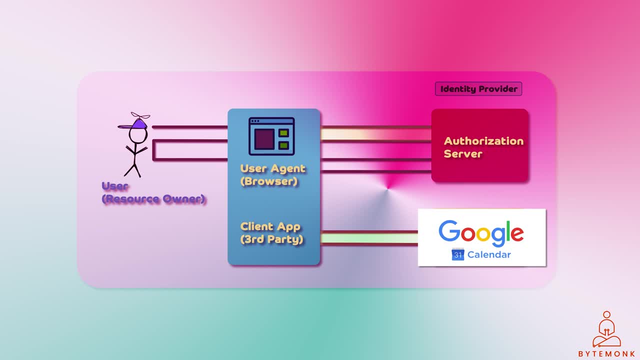 OAuth 2.0 authorization framework. The authorization server is responsible for issuing access tokens and the identity provider is responsible for authenticating users. In some OAuth 2.0 flows, these roles can be combined into a single entity, but in other cases they may be separate entities. 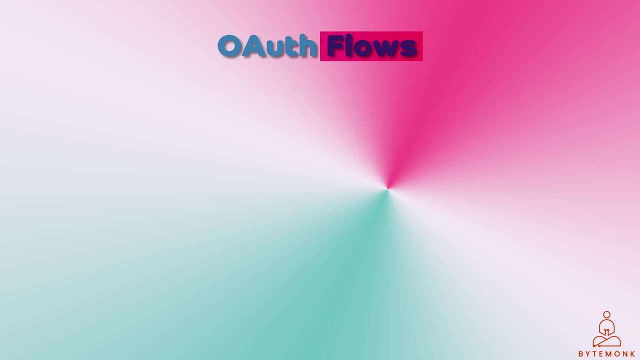 So let's talk about flows. There are four types of OAuth 2.0 flows. Authorization code flow is the most common flow. It is used when the application needs to access protected resources on behalf of the user. The user first authenticates with the IDP. 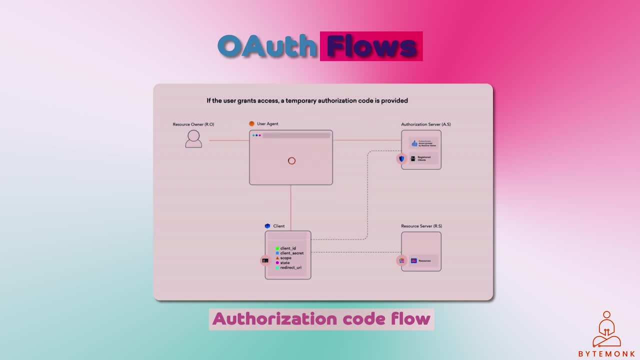 and then the IDP redirects the user back to the application with an authorization code. The application then sends the authorization code to the authorization server, which validates the code and returns an access token and a refresh token to the application. The application can then use the access token to make requests to the resource server. 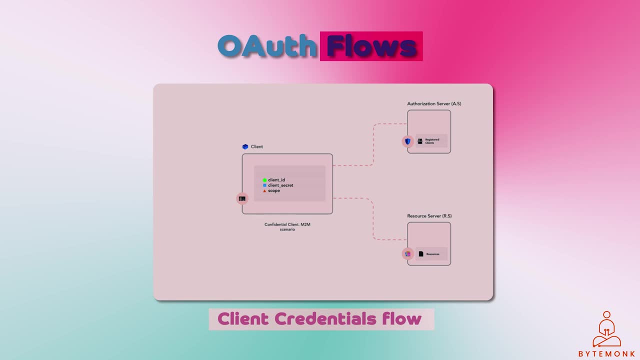 Client credential flows is used when the application does not access protected resources on behalf of the user. Instead, the application needs to access its own protected resources. The application authenticates with the authorization server using its client ID and client secret, and the authorization server returns an access token to the application. 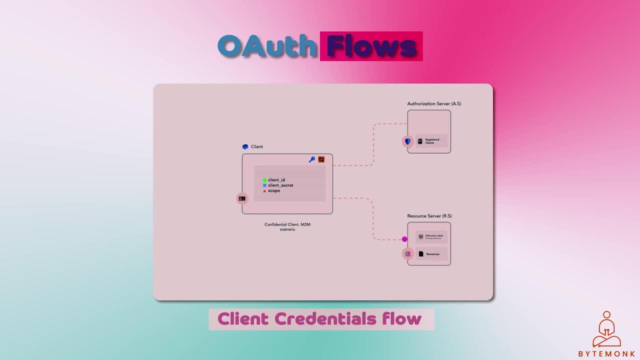 The application can then use the access token to make requests to its resource server. Resource owner. password flow is used when the application needs to access the user's protected resources, but the users do not want to be redirected to the IDP. Instead, the application asks the user to enter their username. 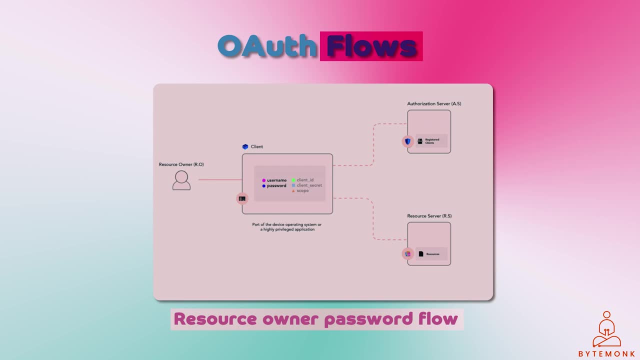 and password directly into the application. The application then sends the username and password to the authorization server, which validates the credentials and returns an access token and a refresh token to the application. The application can then use the access token to make requests to the resource. 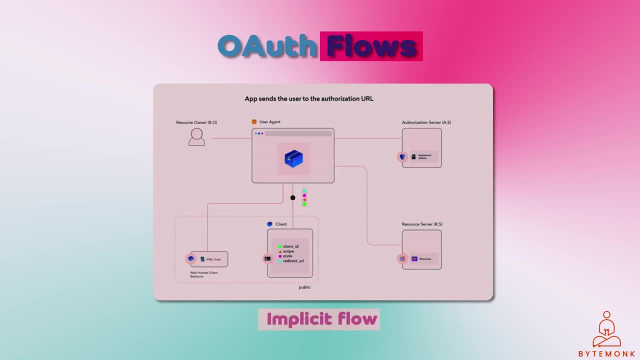 server. Implicit flow is a simplified version of authorization code flow. In the implicit flow, the authorization server redirects the user back to the application with an access token in the URL. The application can then use the access token to make request to the resource server. The implicit flow is not as secure as the authorization code flow. 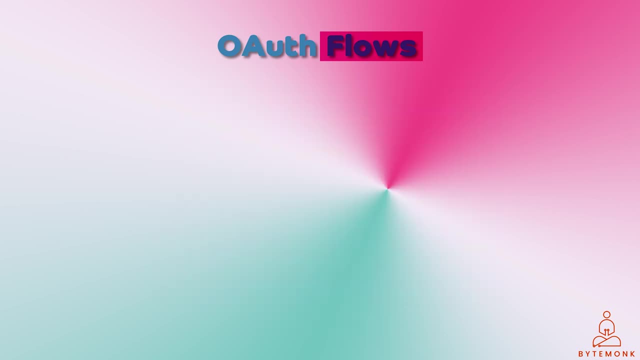 and it is not recommended for most applications. The OAuth 2.0 authorization framework provides a variety of flows to meet the needs of the different applications. The best flow to use depends on the specific application and its requirements, And there is no official OAuth. 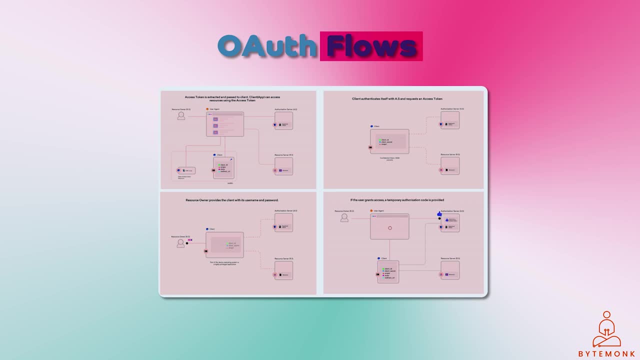 3.0 specification yet, but there are some proposals which are still in the early stages. OAuth 2.0 is currently the de facto standard for authorization in the world of web applications and it is likely to continue to evolve and improve in the years to come.